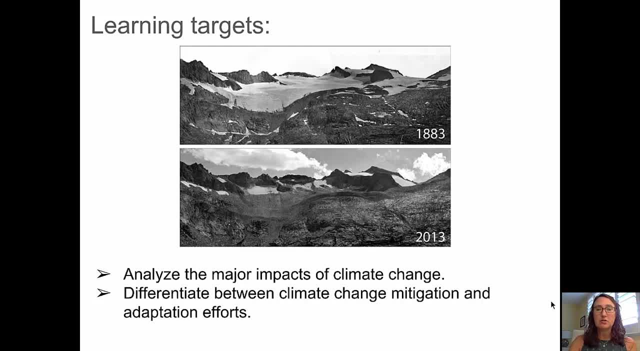 and to differentiate between climate change mitigation and adaptation efforts. I want to call your attention first of all to this picture. We see a before and after picture here, one from 1883 showing a glacial front coming down mountains in Alaska, and the same shot from 2013.. 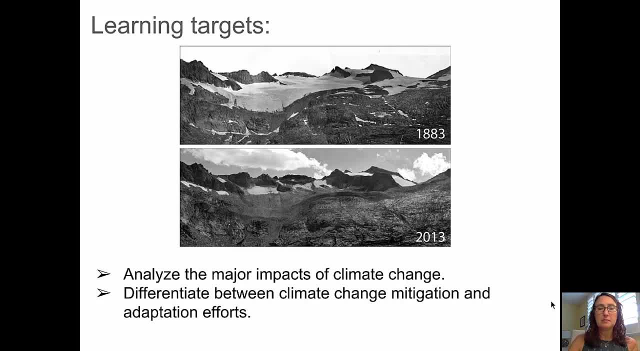 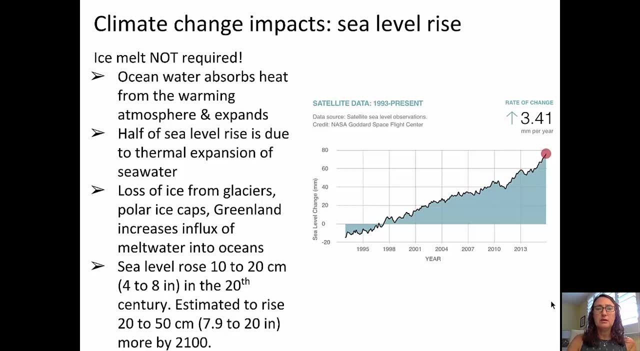 And I think you can clearly see how much this glacier has melted back. Impacts of climate change include things like sea level rise, And for sea level rise we don't really need that much ice melting. In fact, ocean water absorbs heat from the warming atmosphere. 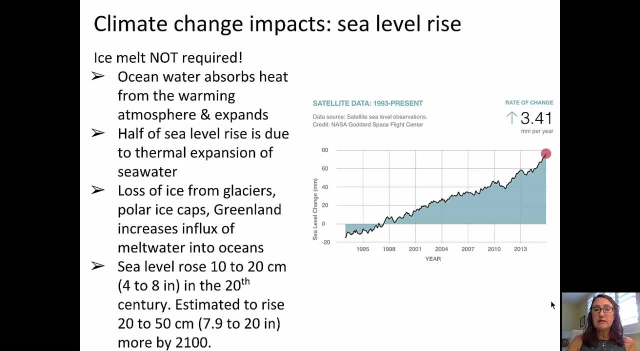 and as it does, it expands. Half of the sea level rise is due to the thermal expansion of seawater. Yes, it's true that the loss of ice from glaciers, polar ice caps, Greenland- increases the influx of melt water into the oceans, and that sea levels rose 10 to 20 centimeters in the 20th century. 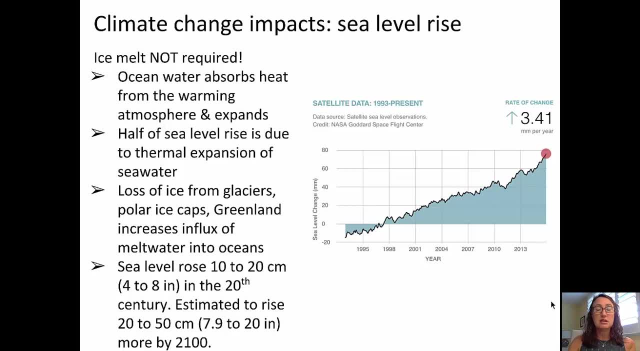 but there's an estimated rise of 20 to 50 centimeters additional by 2100.. Let's look at some data here from NASA Goddard Flight Space Center In the year from about 1990 through till about 2016,. 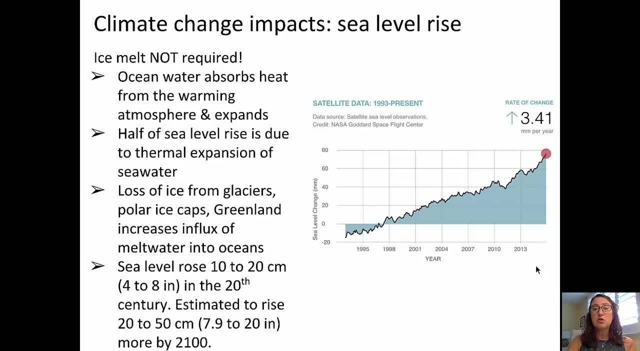 we've seen a rate of fall of about 1.5 percent. We've seen a rate of fall of about 1.5 percent. We've seen a rate of fall of about 1.5 percent. We've seen a change of about 3.41 millimeters per year in sea level. 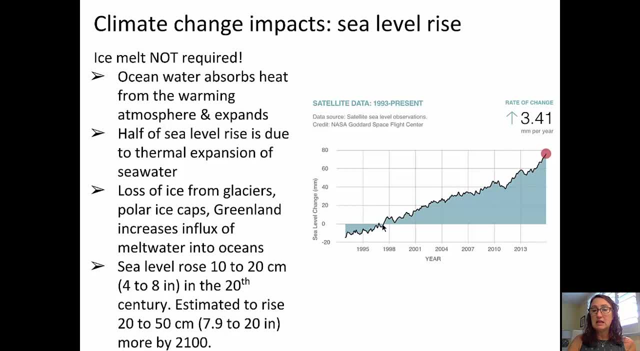 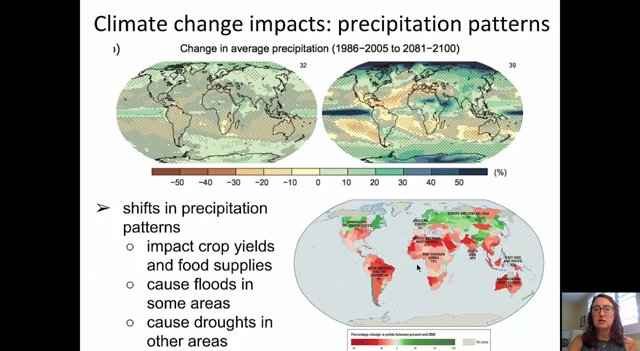 So here is the zero line. Prior to about 1996, sea level was actually below the average, And now, since 1996, we've seen a steady increase in sea level to today's location. Further data comes from precipitation patterns which are being disrupted. In fact, precipitation 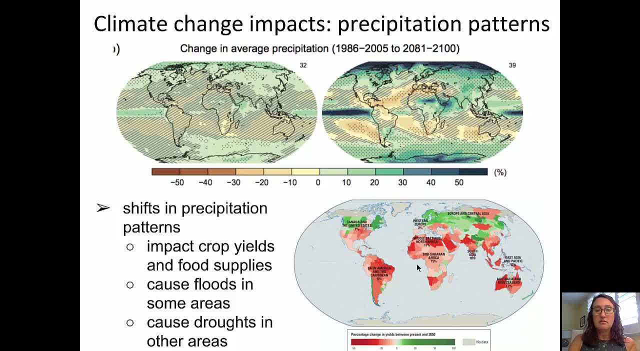 pattern shifts impact crop yields and food supplies. They cause floods in some areas while causing drought. In fact, precipitation pattern shifts: impact crop yields and food supplies. In fact, precipitation pattern shifts impact crop yields and food supplies. In fact, precipitation pattern shifts: impact crop yields and food supplies. 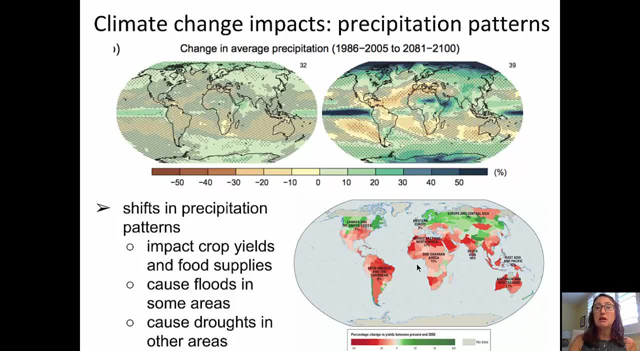 In the top diagram we can see the average precipitation compared between the years 1986 to 2005 on the left and the year's projections for 2081 to 2100 on the right. The zero mark is here in the middle. Anything that's in a green or a blue color would indicate. 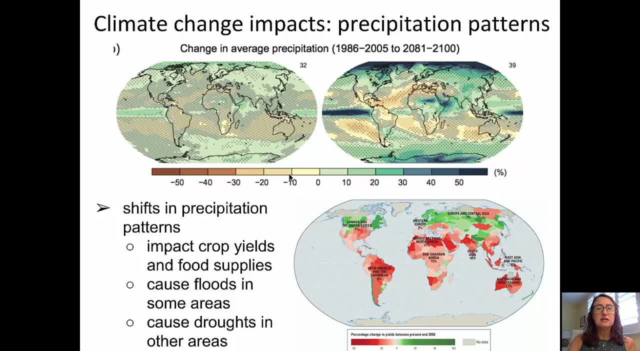 an increase in precipitation in that region. Anything that's in a tan or a brown color would indicate a decrease in precipitation in that region. So we can see that the patterns change from past years through to the future and they don't change regularly across the globe. 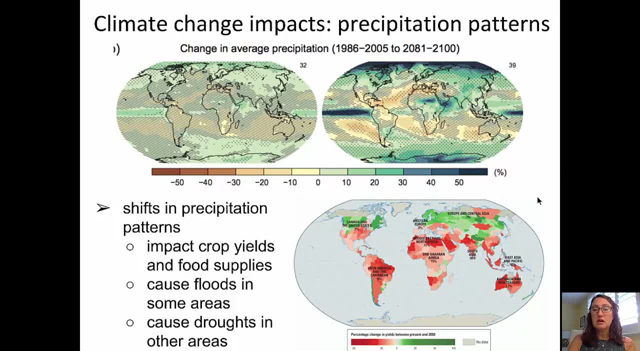 In the bottom diagram we can see how that might play out in terms of crop yields between now and the year 2050.. So, as you might expect, green is good. here Go go Lots of crops growing And you can see few areas indicated in green where we're expecting an increase in crop yields. 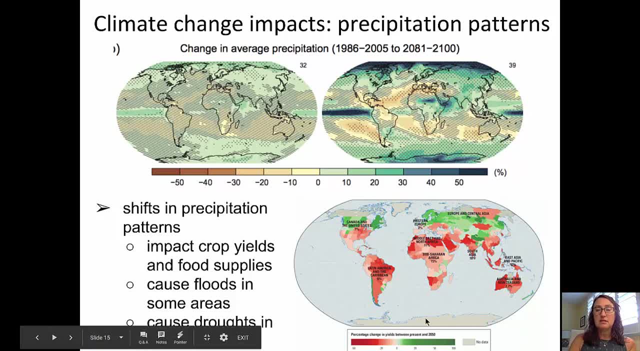 But in the red we're expecting decreases in crop yields. So think about where populations are increasing the most and think about how that pattern might play out in terms of food supplies. Further evidence of the impacts of climate change come from ice, First of all. 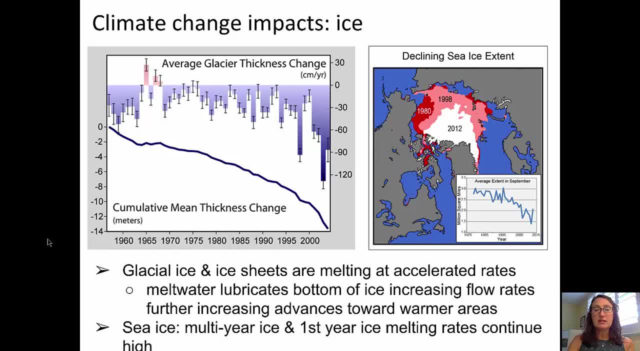 glacial ice and ice sheets are melting at accelerated rates And that melt water can actually lubricate the bottom of the ice, which increases the rate that it flows, which causes some of that ice to move towards warmer areas where it melts more rapidly. 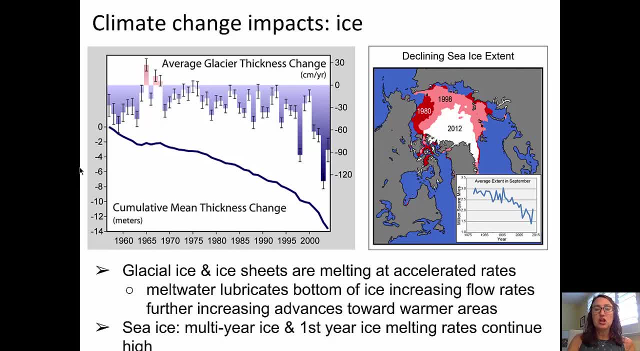 And we're seeing evidence of that in the cumulative mean thickness change graph here. So from the year 1955 up to the year 2005, we can see a steady decline until about 1995 when the decline increased. The slope became steeper here. In terms of sea ice, we're seeing declines in both. 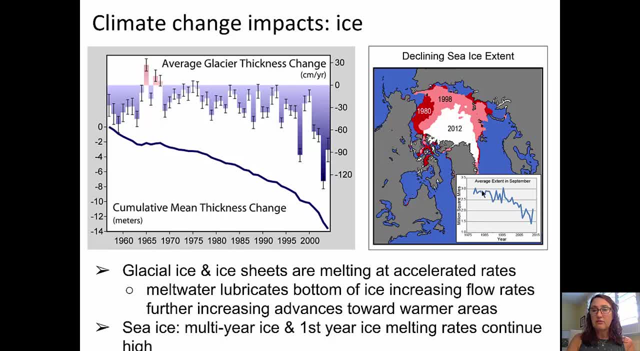 multi-year ice and first-year ice And you can see the graph here indicating the extent of sea ice in September. So September is a key time because it's the end of the melting season in the Arctic. So this would be minimum sea ice values If you look at the outline of the red area. 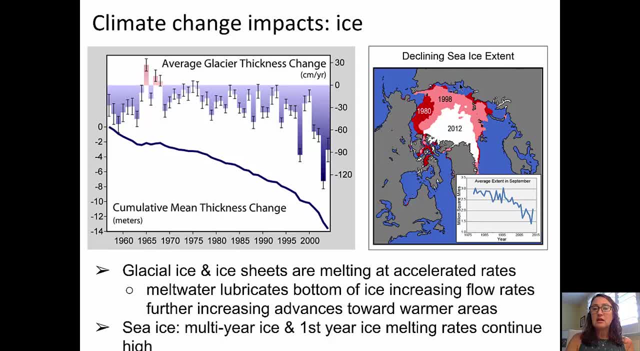 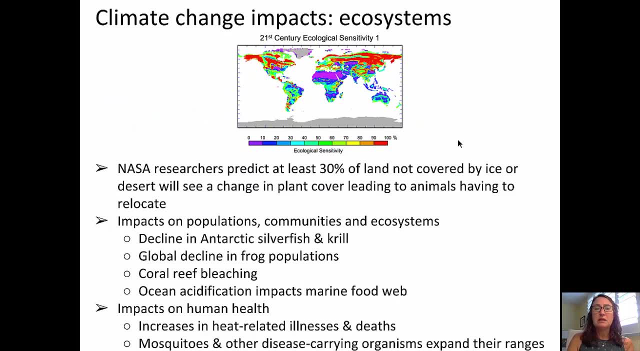 that's the 1980 extent of sea ice And compare that to the dramatic reduction in 2012.. Turning now to talking about ecosystems and how they have been impacted by climate change. In fact, NASA researchers predict that at least 30% of land not covered by ice or deserts will see a change in. 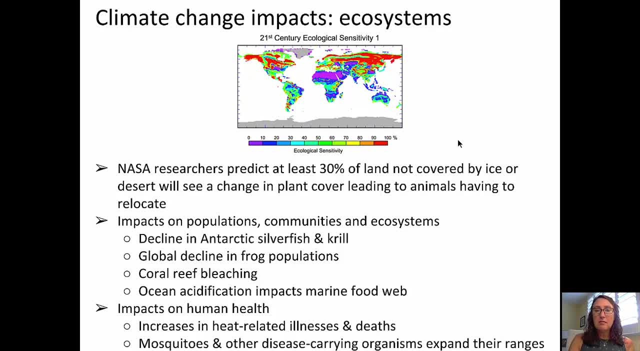 plant cover, which is a significant increase in the amount of land covered by ice. So that's a significant increase in the amount of land covered by ice, So that's a significant increase in the animals having to relocate, And that impact on populations includes things like declines in.